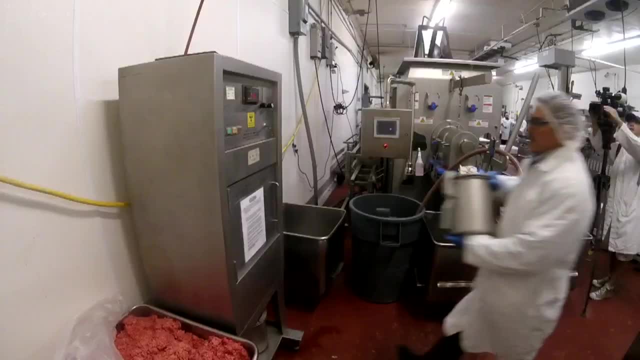 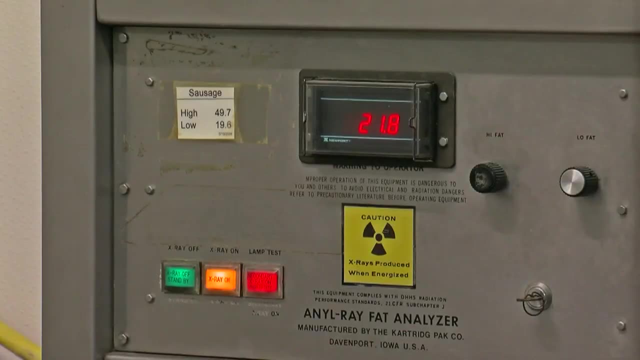 It's actually an X, This ray. the ray is a light beam that goes through the beef, which gives us an instant fat content versus lean. It gave us the answer in seconds. Are you always within .1 or .2%? We try to be. 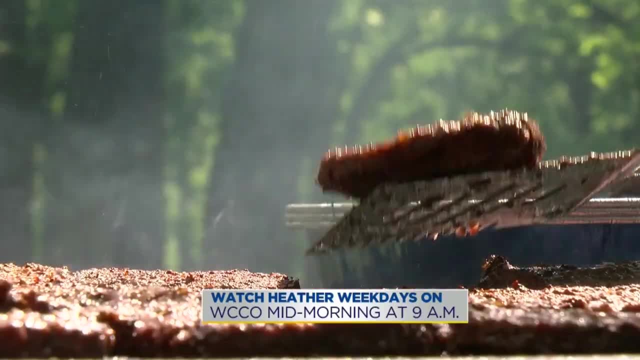 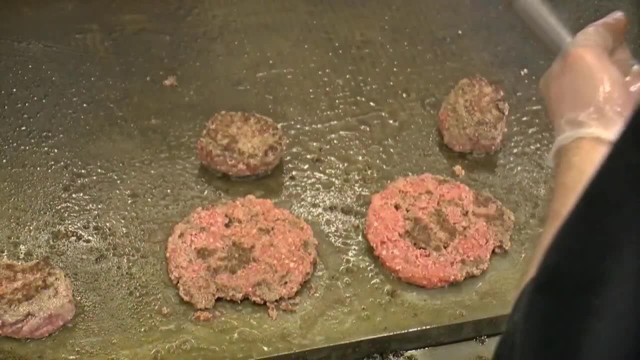 Mann recommends the 80% or 85% lean for your backyard grill. That'll avoid flare-ups, So you would not have a forest fire. And in the mid-70s, when you're eating out, 70% lean is the lowest allowed by law. 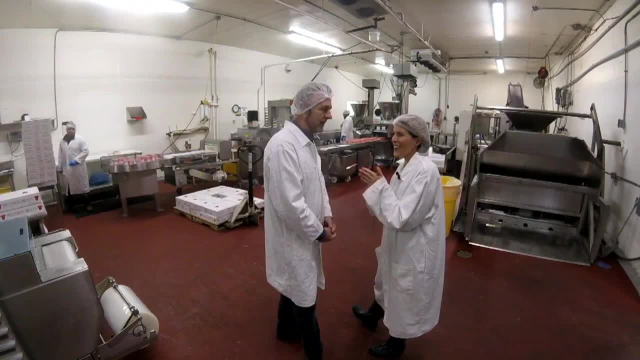 You're telling us don't be afraid of the 70%. Nope, Don't be afraid. Don't be afraid of it because your heart doctor wouldn't tell you to do it, but your taste buds would tell you to do it. WCCO 4 News. 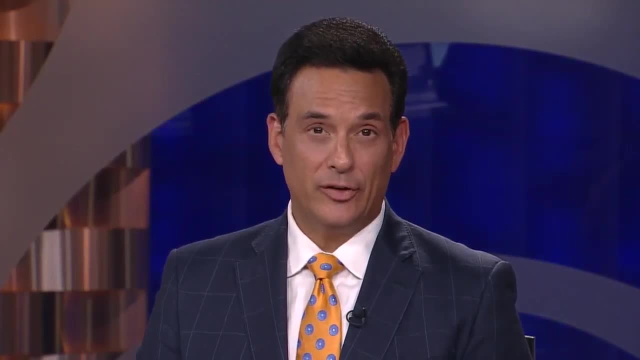 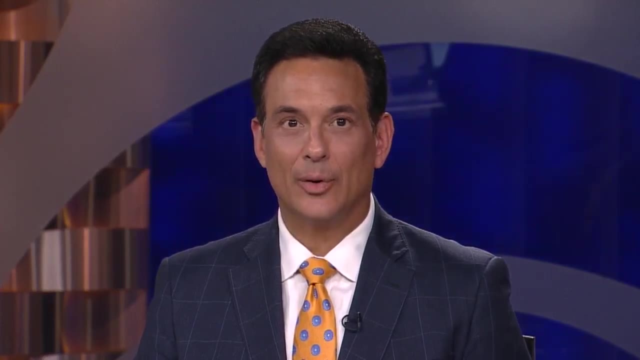 The USDA regulates ground beef labeling At Swanson Meats. a USDA rep is actually on site and does some daily spot checks. One thing she checks on is the lean content of the ground beef. Share your good questions with Heather on Facebook or on Twitter. 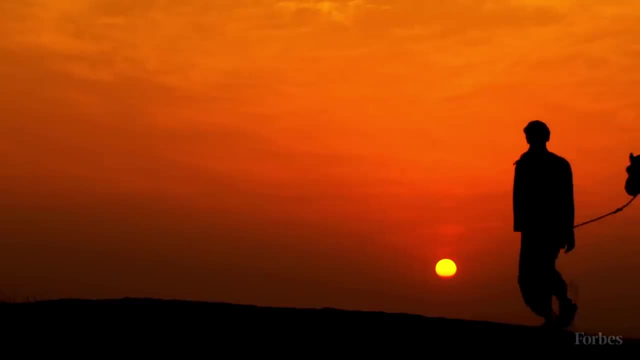 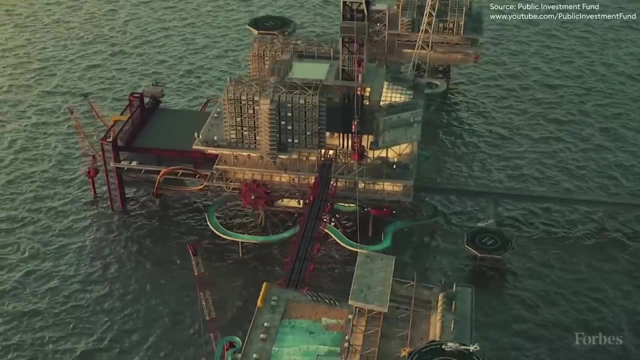 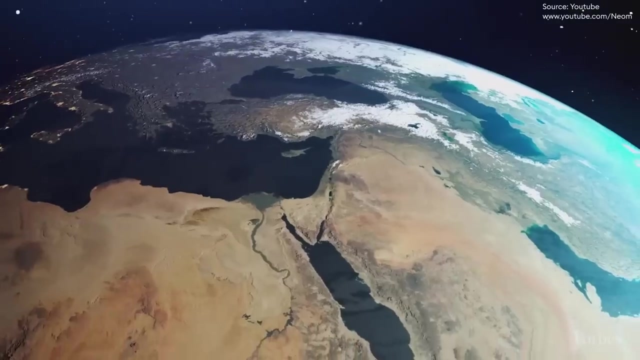 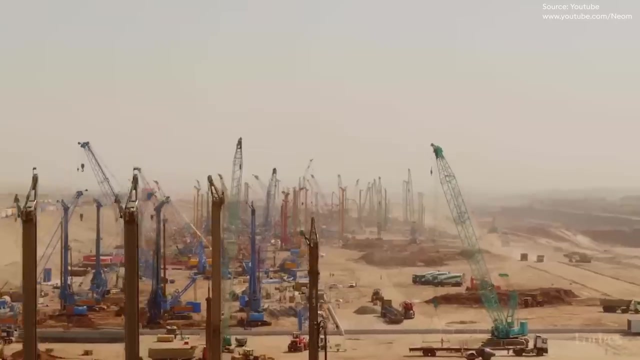 Saudi Arabia is on a massive building spree, creating private islands, luxury hotels, theme parks, cruise ports and even a desert ski resort. The question remains: if they build it, who will come? Whatever your preconceived notion of Saudi Arabia as a travel destination is, it's about. to get a major renovation. Imagine Sindala, a seven-star private island resort with three ultra-luxe hotels, 38 high-end restaurants and multiple superyacht marinas. Or Qadiyah, a futuristic city of 600,000 people rising from the desert floor dedicated to esports. 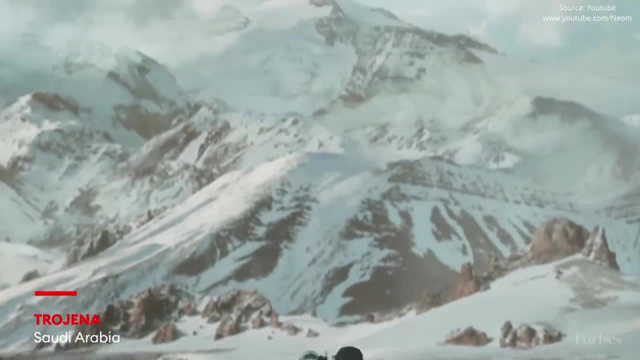 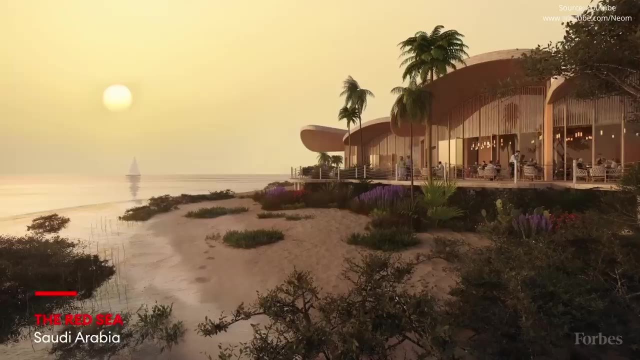 and gaming. How about Trojana, a space-age ski resort built above the high desert Or the Red Sea, a vast waterscape of 50 luxury resorts and 8,000 hotel rooms spread across 22 islands in a Maldives-style archipelago powered entirely by wind and 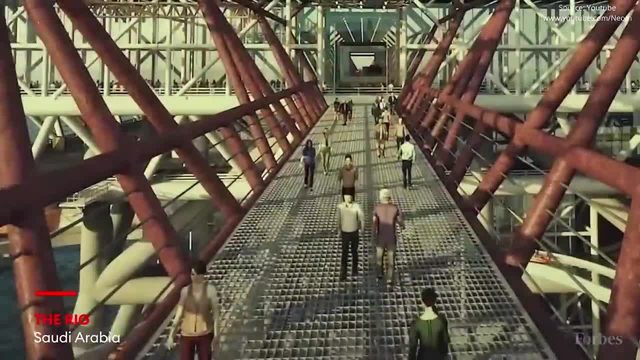 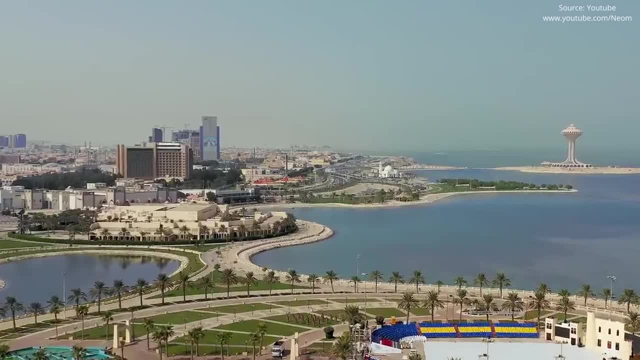 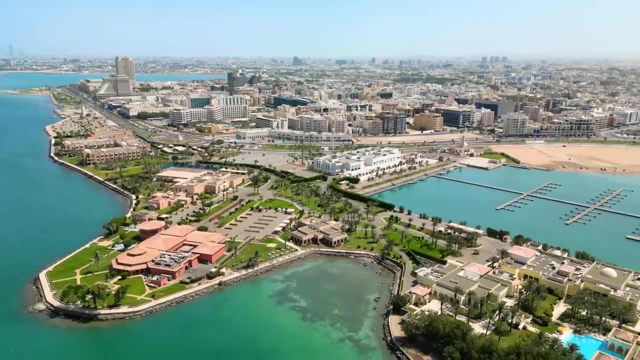 solar energy. Also in the works is The Rig, a $5 billion adventure theme park built on an offshore oil platform. In addition, Saudi Arabia is positioning itself as a major cruise destination, with Cruise Saudi having recently bought a $300 million ship.